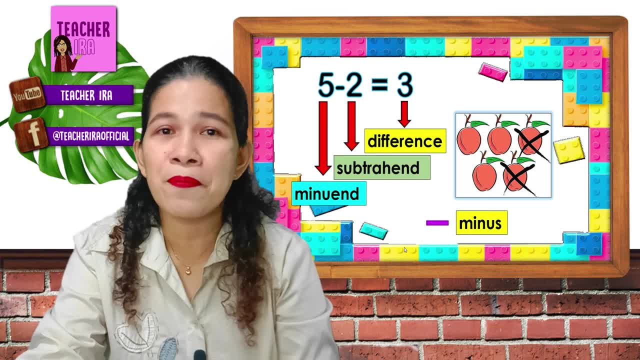 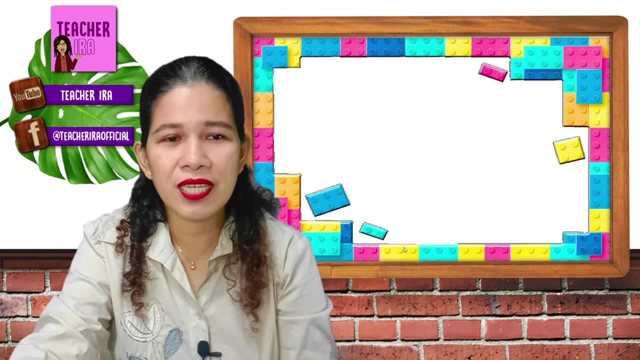 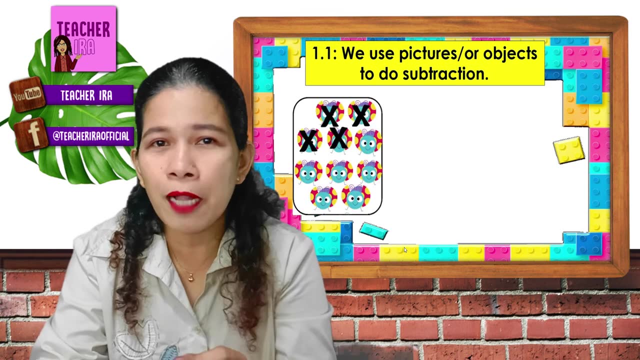 And the symbol that you will use here is minus. You say minus. Now let me tell you and let me teach you the different ways and how to do subtraction. First, we use pictures or objects to do subtraction. So I have here pictures and this will help us a lot in subtraction. 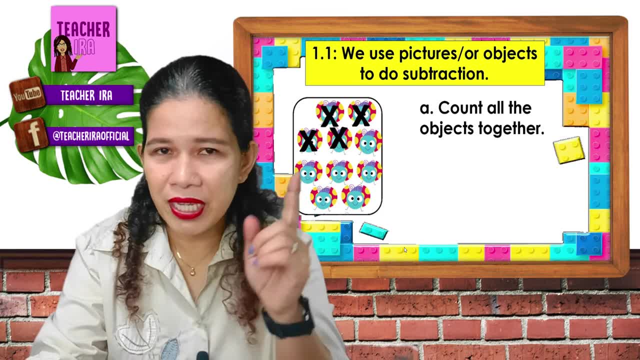 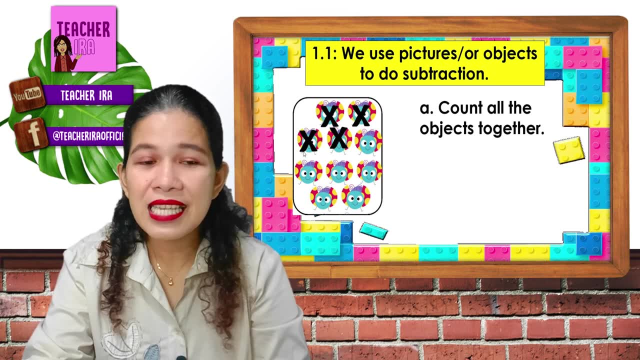 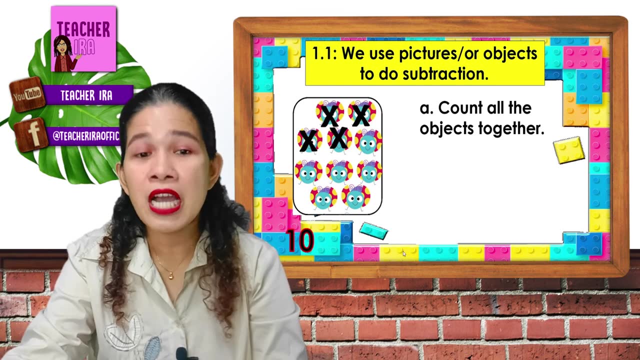 What are you going to do? First, count all the objects together. Now let us count all the numbers that we have here, All the objects One, two, three, four, five, six, seven, eight, nine, ten. So there are ten objects that we have here. Now count all the objects with. 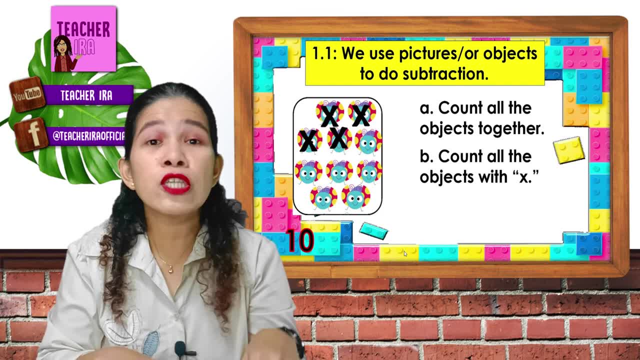 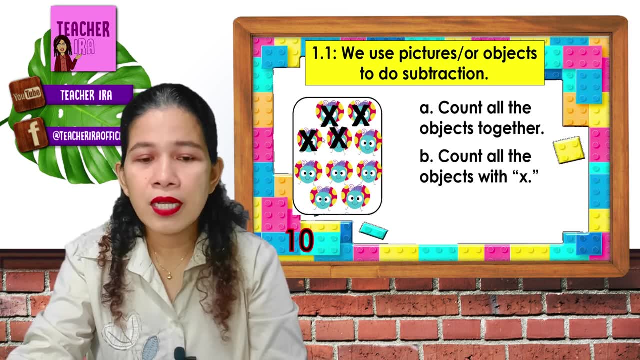 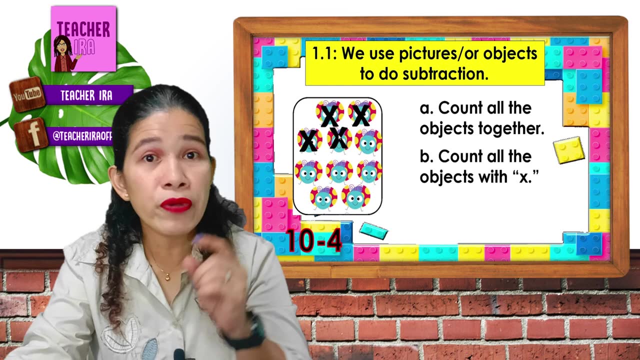 x. So the next one, next procedure is you find all the objects with x and you count them. Let's count One, two, three, four, five, six, seven, eight, nine, ten. So there three, four, So there were four, So you would say ten minus four. So out of this ten you will remove. 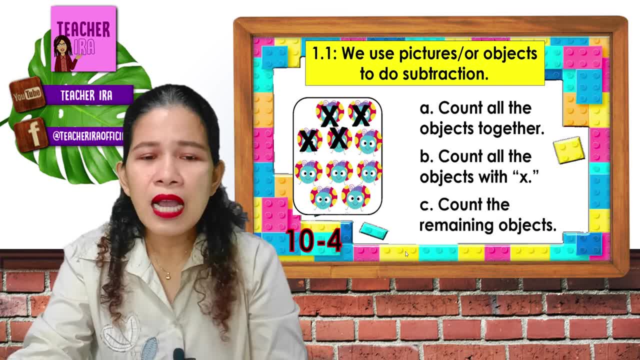 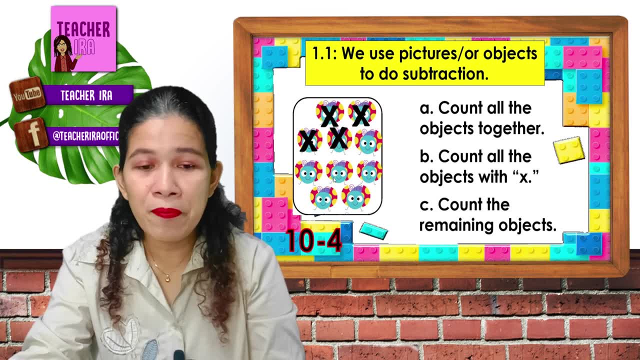 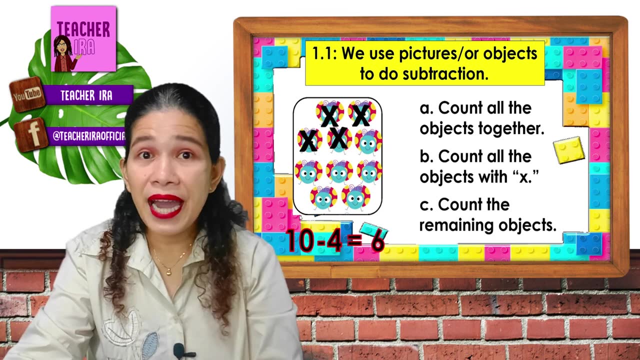 the four. Now what's gonna be the answer? Count the remaining objects. Let us count One, two, three, four, five, six. So the remaining objects are six. Therefore, that is the difference or the answer. So you would say ten minus four equals six. Next, we use pictures or objects to do 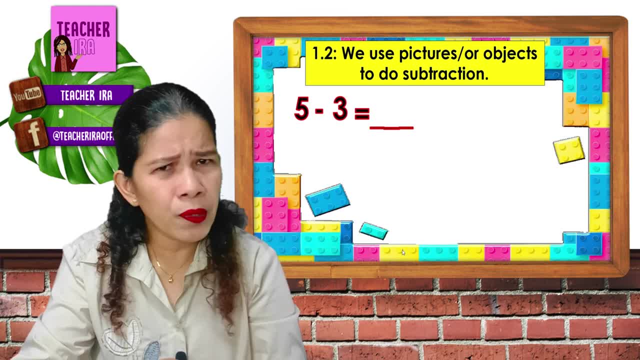 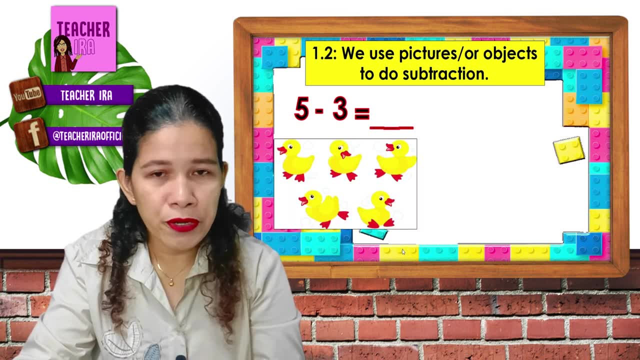 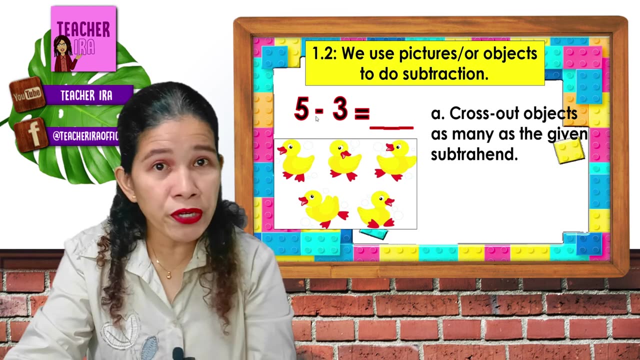 subtraction Five minus three equals what's gonna be the answer. So here we don't have x's, yet We have pictures. So what are you going to do? First, cross out objects as many as the given subtrahend. So the subtrahend that we have here is a smaller number, which is three. So we're going. 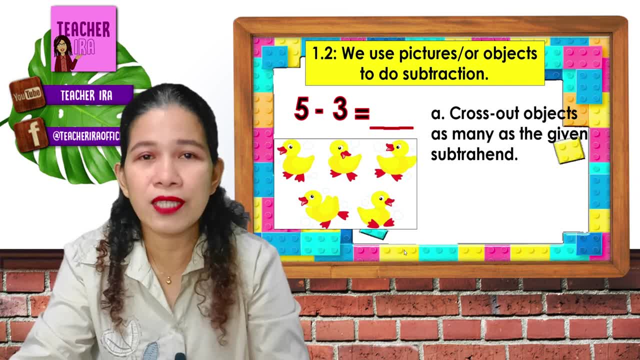 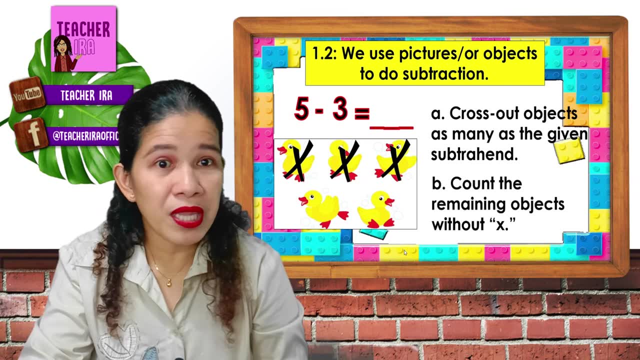 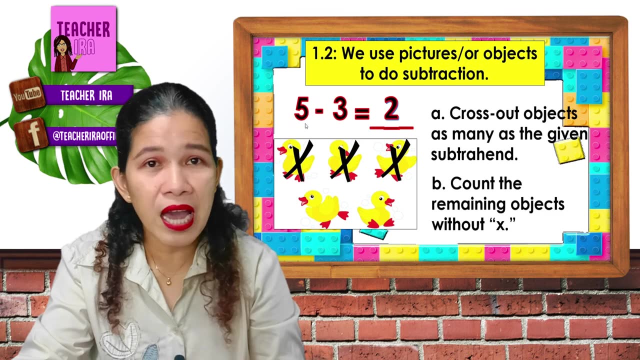 to cross out three objects Among the five dots. Let's do it: One, two and three. Now count the remaining objects without x, That is two, One, two. So that's gonna be your answer. So you would say: five minus three equals two. 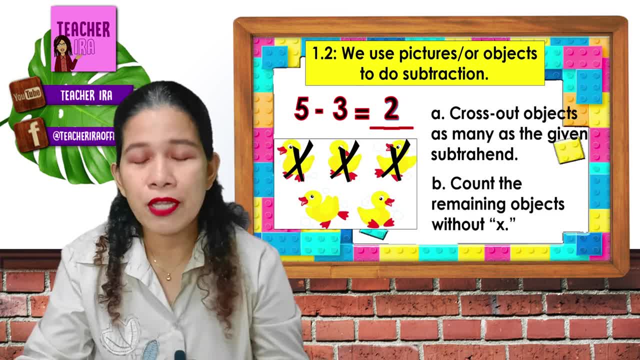 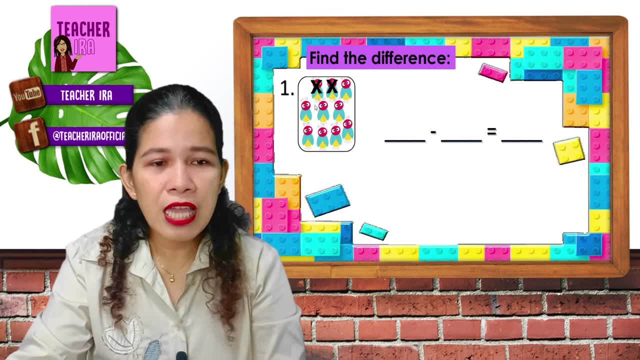 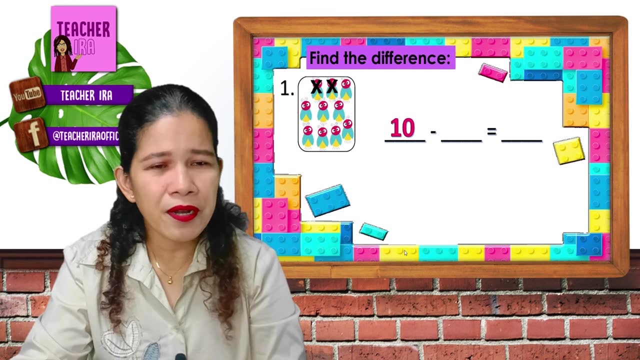 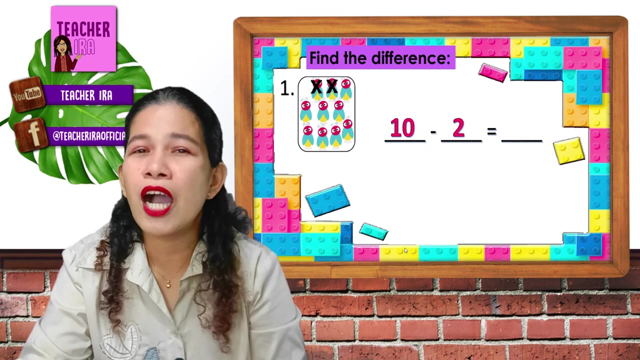 So it became easy because of the objects that we used. Now let us try Find the difference. Let us count the objects first: One, two, three, four, five, six, seven, eight, nine, ten. So there are ten objects. And how many x's were there? One, two, Okay, So you write two. That says ten minus two. 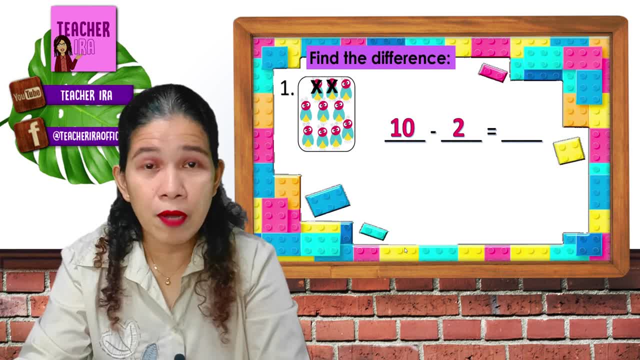 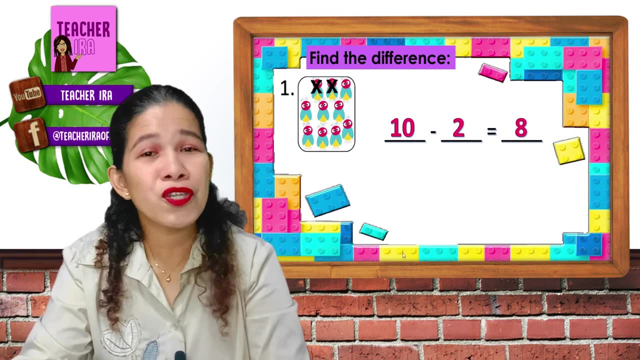 How will you find the answer? Very good. Count the remaining objects without x: One, two, three, four, five, six, seven, eight. So your answer is eight. So you would say ten minus two equals eight. Great job, Number two. 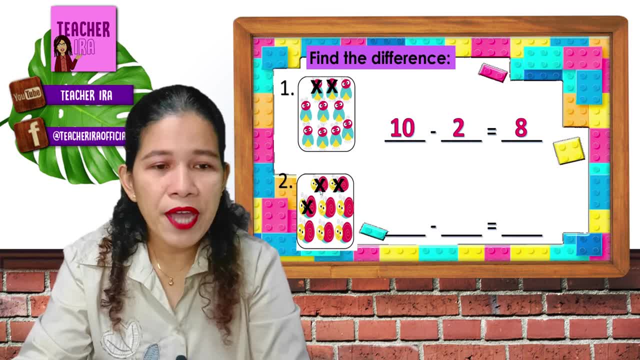 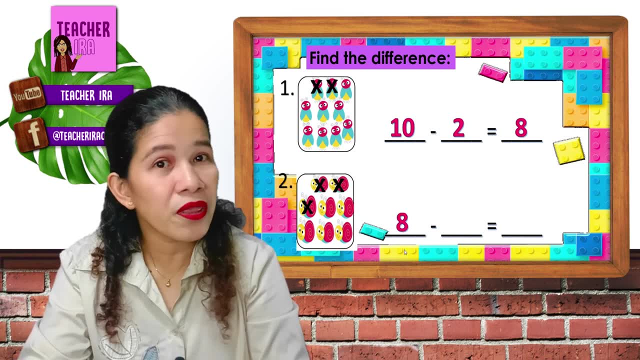 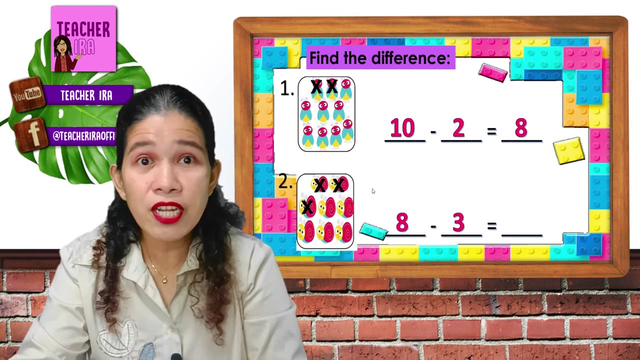 Let's count all the objects together: One, two, three, four, five, six, seven, eight, So you got there eight. And then count all the x: One, two, three, So you got three. That says eight minus three. 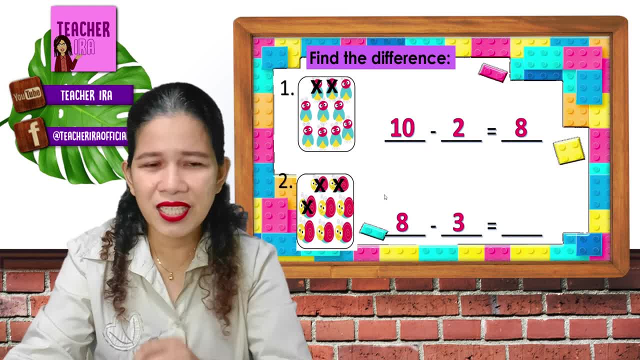 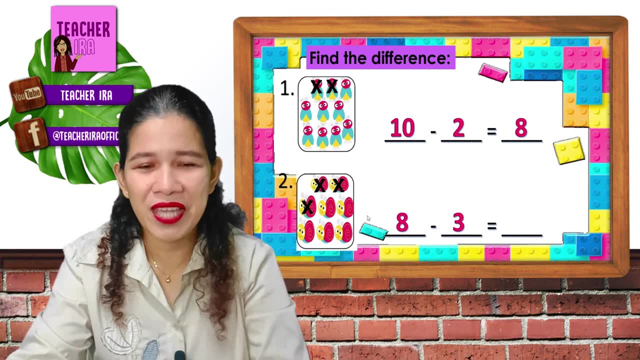 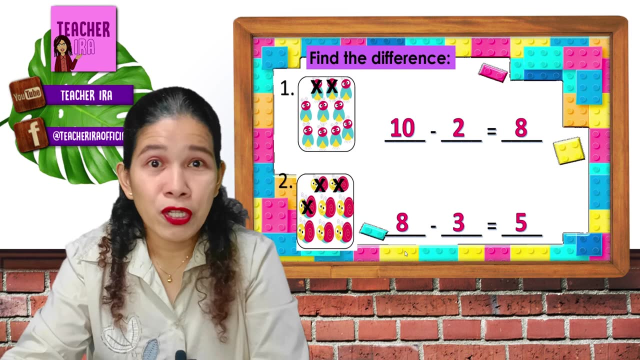 Now, how will you find the answer Correct? again, Count all the objects without x: One, two, three, four, five. So the answer is 5.. Very good children, We are getting it now. Now I'll show you some more ways of doing subtraction. 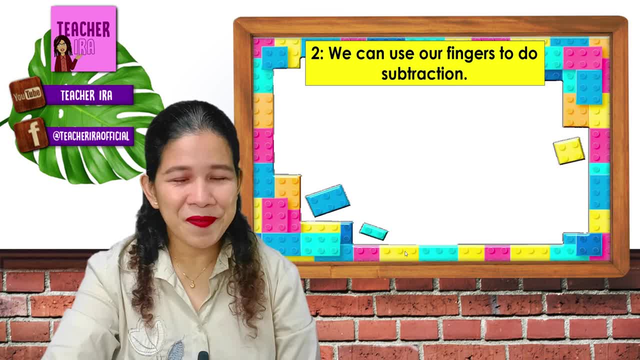 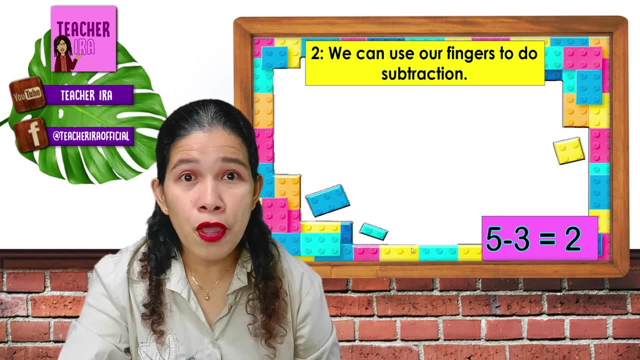 Number 2.. We can use our fingers to do subtraction. Wow, That's gonna be exciting. So get ready with your fingers now, kids. So let's have 5 minus 3 equals 2.. We're going to find the answer using our fingers. 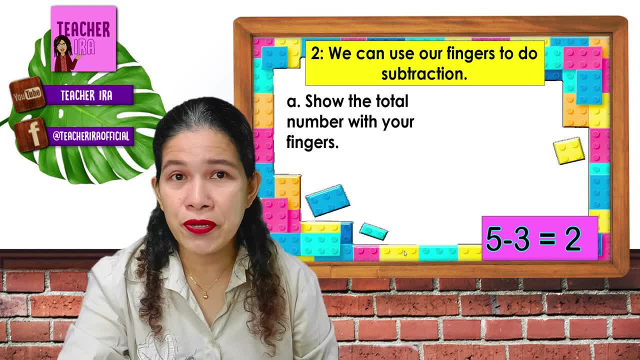 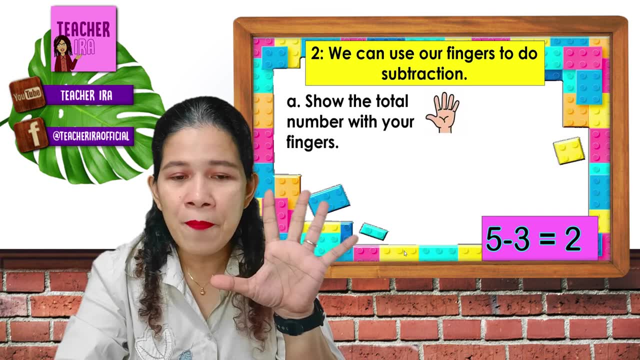 First show the total numbers with your fingers. So let us have 5.. That's gonna be the minuend, So you have to show all of that. So that's 5.. Now, next step: Fold the number of fingers according to the given subtrahend. 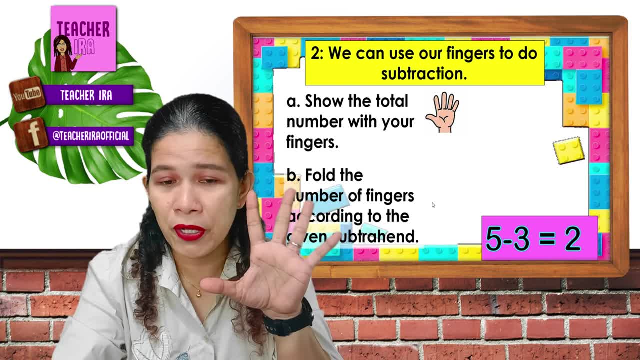 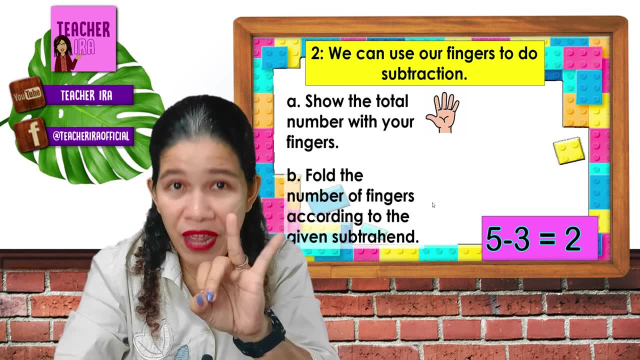 So what is our subtrahend? Very good, That's the smaller number, So we got her 3.. So let's fold 1,, 2, and 3.. Were you able to do it? Very good. 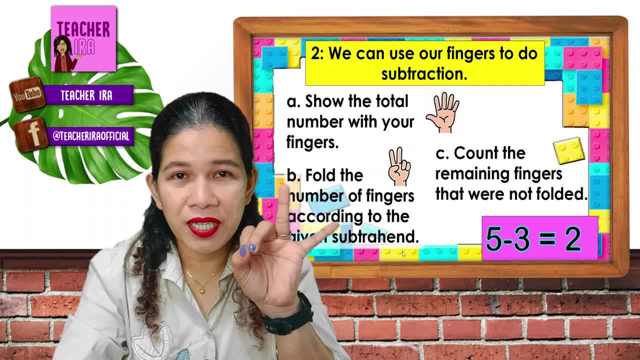 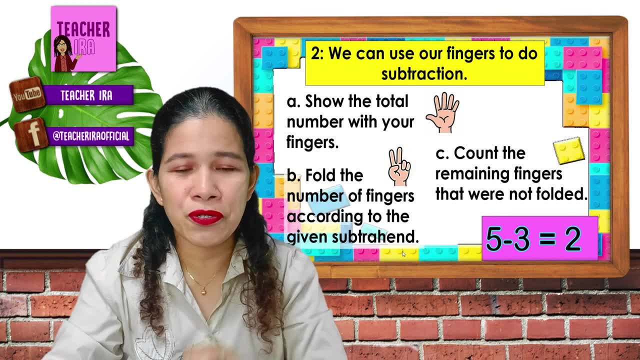 Now count the remaining fingers that were not folded. Let's count 1, 2.. Since 2 fingers were left, that is our answer. So we would say 5 minus 3 equals 2.. It is easier because we used our fingers. 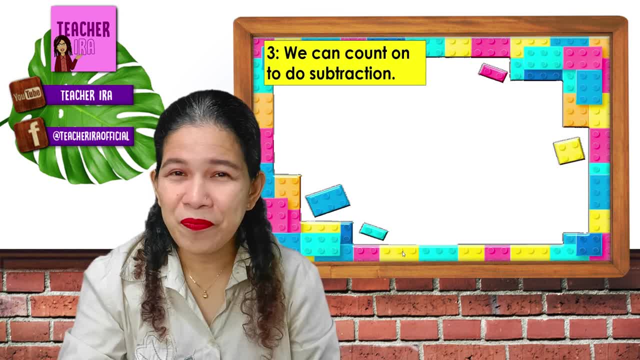 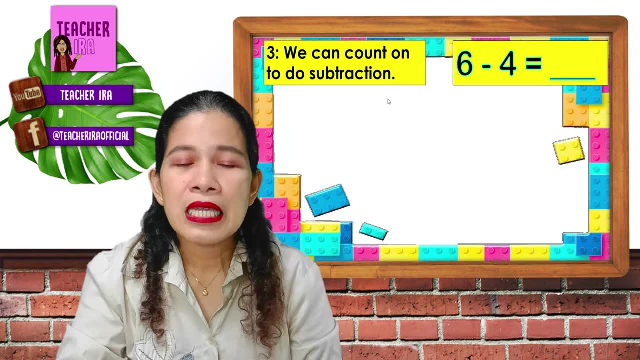 Let us have another one We can count on to do subtraction. Remember, in addition, we did the counting on. We can do that also in subtraction. How? Here is the problem: 6 minus 4.. What's the answer? 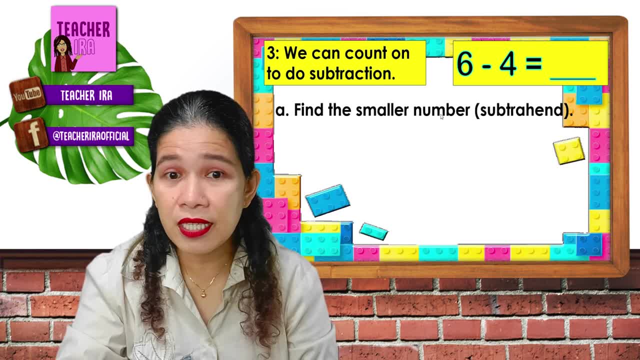 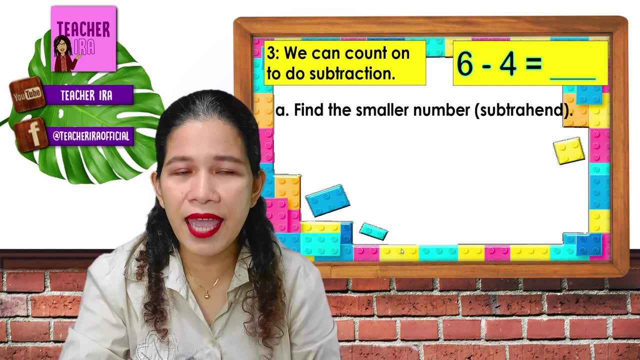 First find the smaller number. So which is smaller? Is it 6 or 4?? Very good, 4 has the smaller value And that is the subtrahend. Next, think of the next number to it and count on. 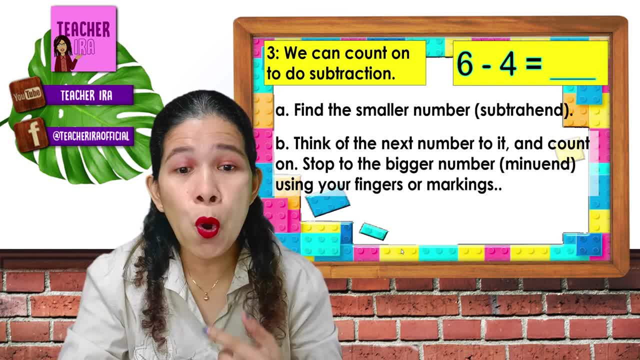 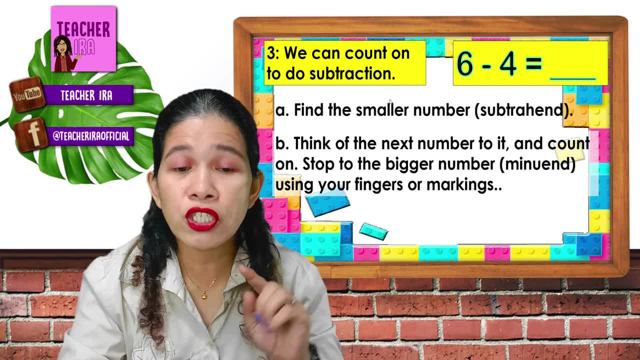 Stop to the bigger number using your fingers or markings. Okay. next, The number of fingers or markings you've used to reach the domino end would be your answer. Let's do it step by step. So the smaller number, The smaller number, is the 4.. 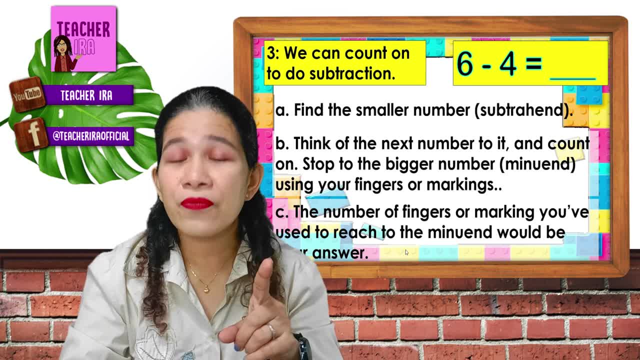 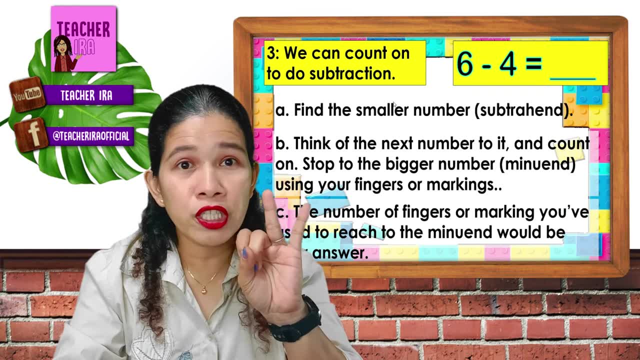 Now think of the next number to number, 4.. That is 5.. Good, 5, and count on 5, 6.. Okay, stop. You will stop until 6, only Then count the number of fingers you've used. 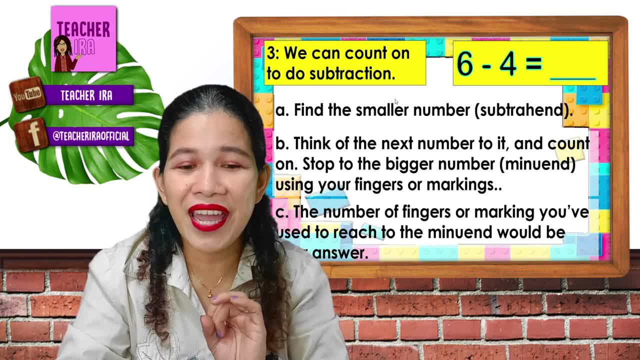 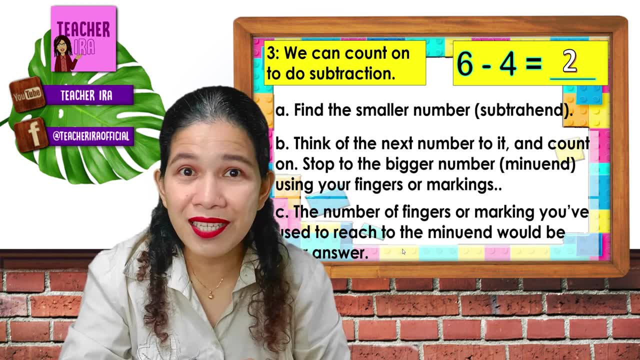 1, 2.. So that's your answer. Easy, We can also use markings like 4,, 5,, 6.. Like dots or lines, And then you are going to count them and that's going to be your answer. 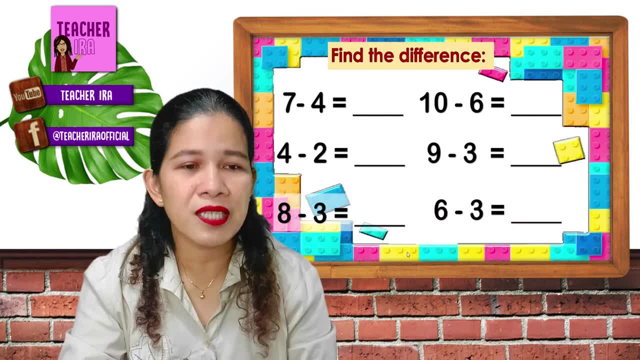 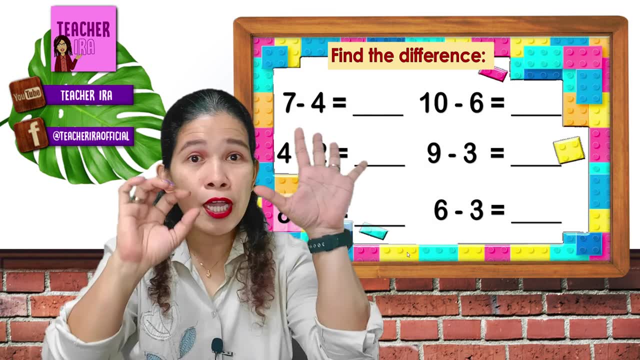 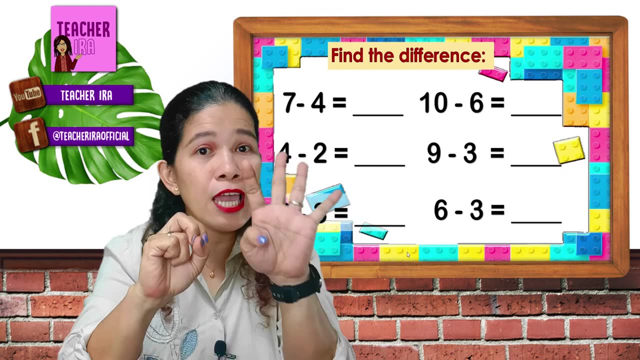 Now let us try that with the following. Find the difference. We use finger folding or counting on. Let's do 7 minus 4.. So we could use finger folding, 7 and let's remove 4.. 1,, 2,, 3,, 4.. 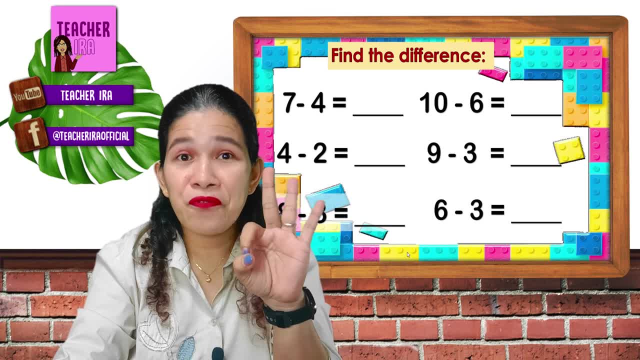 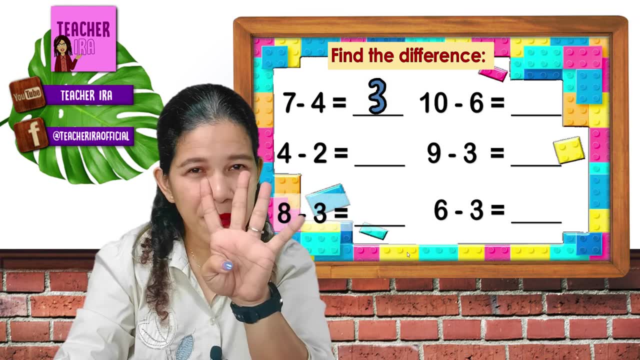 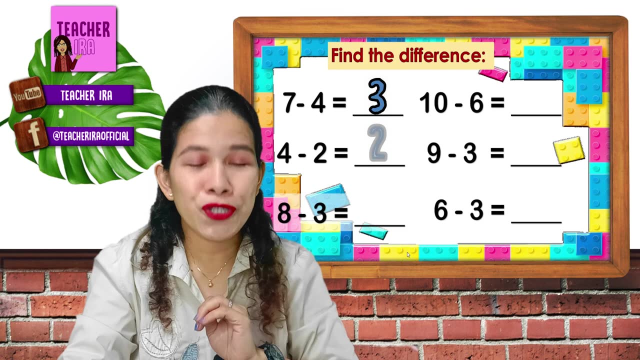 So what's your answer? Very good, That's 3.. How about 4 minus 2?? So you got 4 minus 2.. 1, 2.. So what's the answer? Very good, So that's 2.. 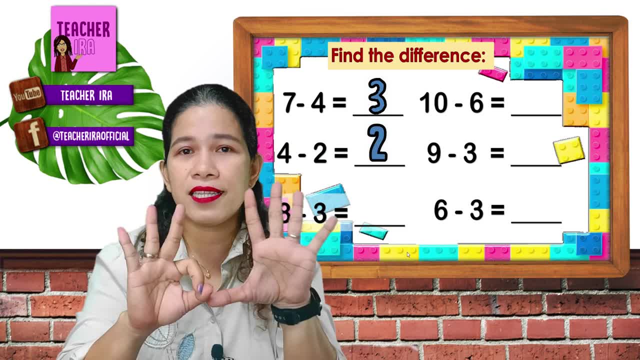 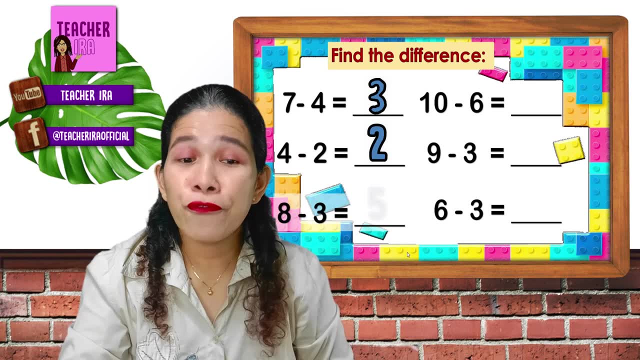 8 minus 3.. So let's have 8.. 8 minus 3.. 1,, 2, 3.. So what's your answer? Great, It's 5.. Easy, Wow, you are getting it now, kids. 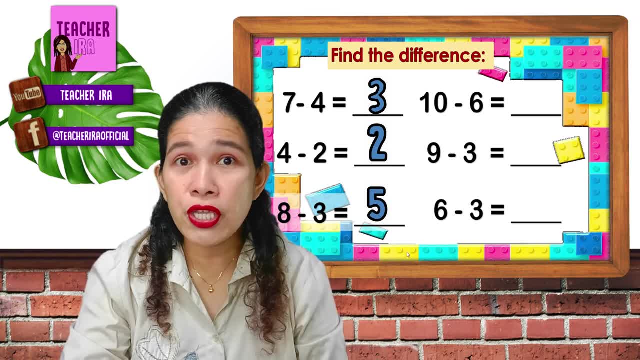 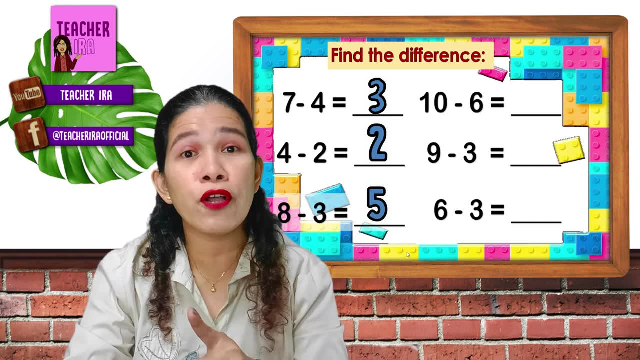 Now with this 3, let's try to use the counting on. So which is smaller, 10 or 6?? Yes, it's 6.. So let's start from the subtrahend and think of the next number to it.